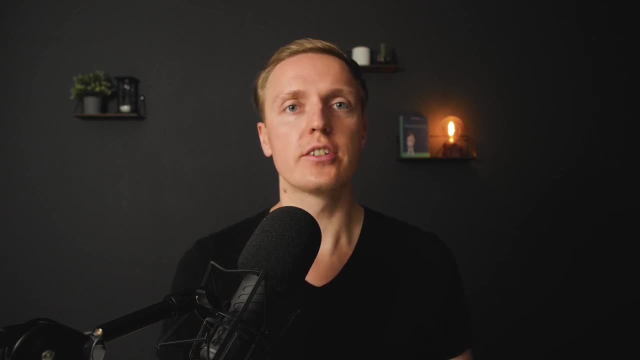 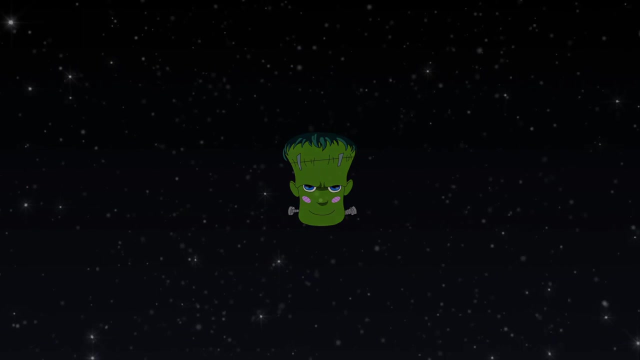 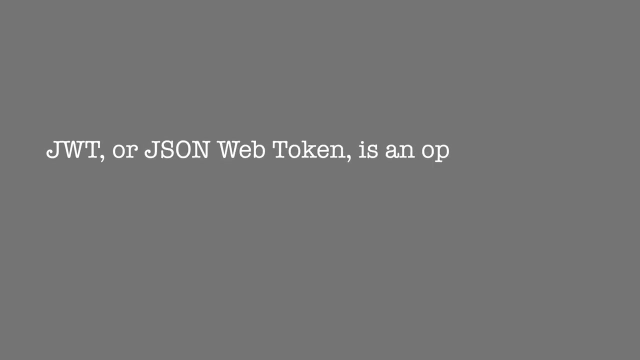 In this video you will learn in a super easy way what is JVT authentication and how we can implement it inside Nodejs. So the first question is: what is JVT authentication and why do we need it at all? And actually it is a most popular way to authenticate an login user inside your web. 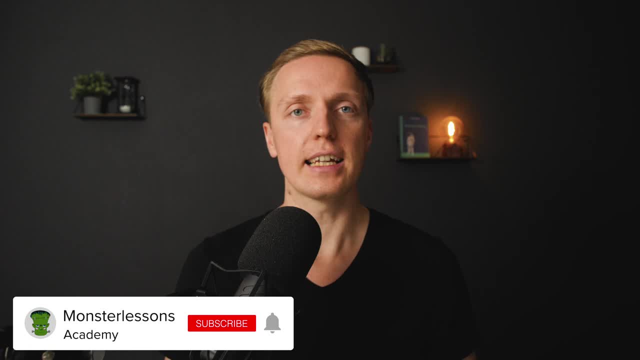 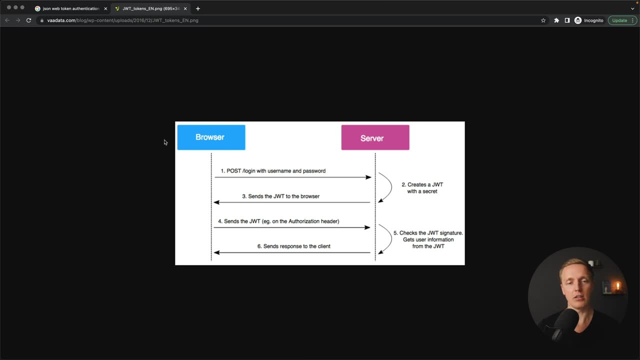 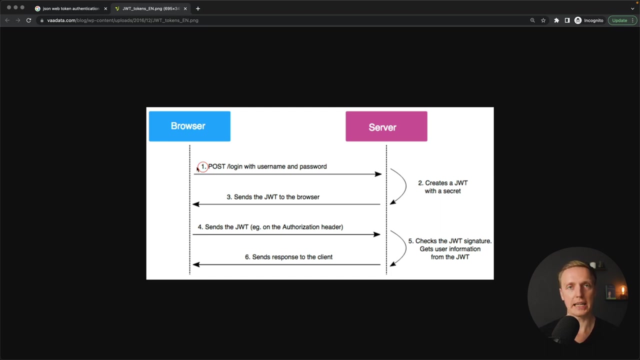 application, And you can use it both with web applications and with mobile applications, And here is how it works. As you can see, we have two different things: Client, or our browser and server, And the first step here is that our client sends a login request to the backend. 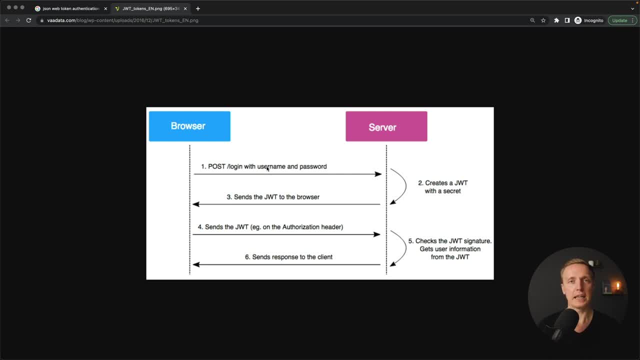 Typically it is an API slash login where we are pasting our username and password. Server checks our credentials, checks that this user exists in the database and generates back not only user information but also a JVT token. So, as you can see here, creates a login request to the backend. And here is how it works. As you can see here, creates 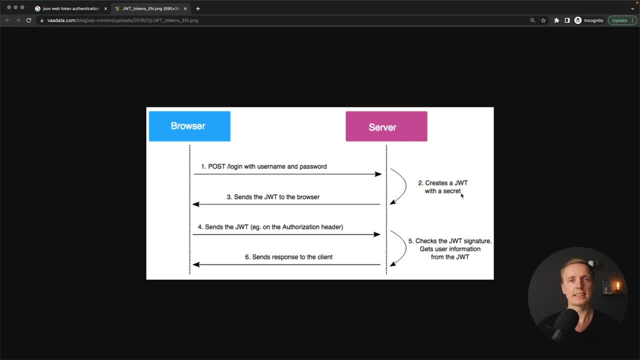 a login request to the backend. And here is how it works, As you can see: here creates a login request to the backend, And here creates a login request to the backend, And here creates a JVT with a secret. So what is JVT? This is just a random string which contains some information. So we are getting on. 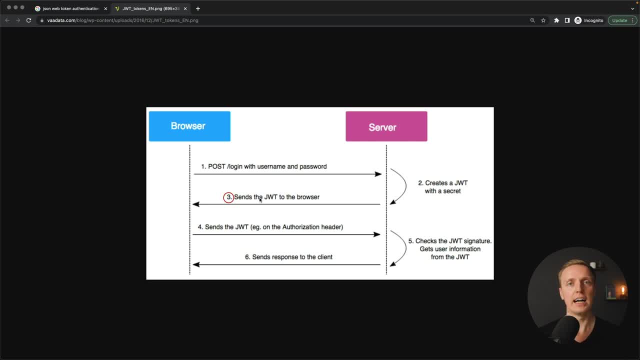 the client this JVT token in the response. After this, the goal of the client is to save this data somewhere, for example in a cookie or in local storage, So somewhere where our client can use it later. So later our client is sending requests to the backend and will typically add this JVT. 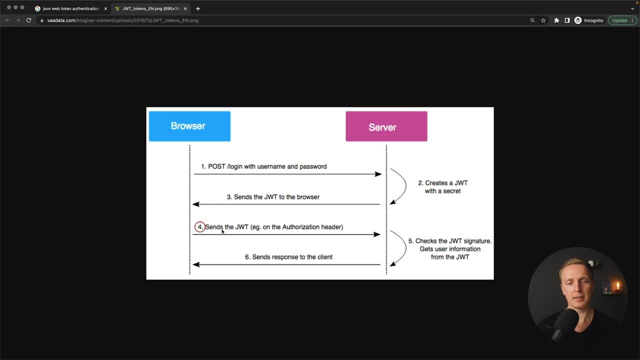 token to all the requests And this is the first step- send a JVT token inside authorization header. So we are adding this JVT token inside our headers And after this our server gets this request, parses our headers and reads the token And it understands to which user this token belongs. 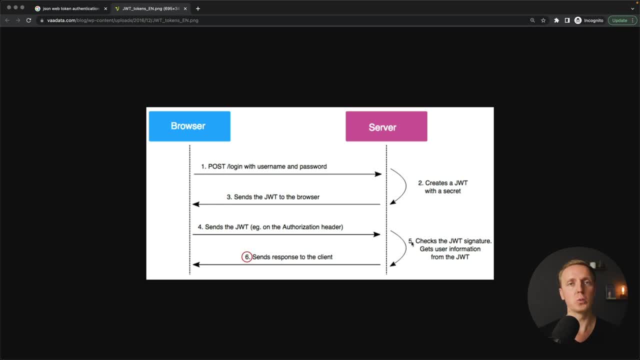 by parsing this token, And after this, our server will deliver correct information to our client. So this is exactly how JVT token works, And after this, our server will deliver correct information to our client. So this is exactly how JVT token works. 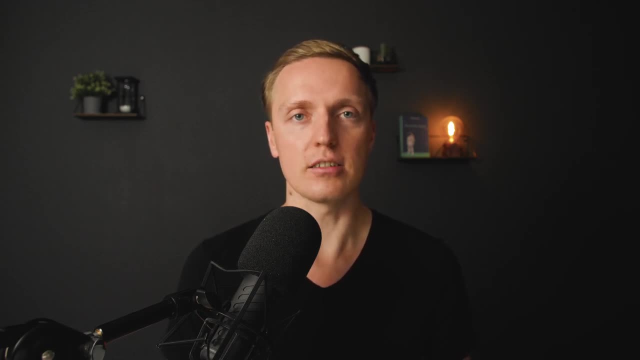 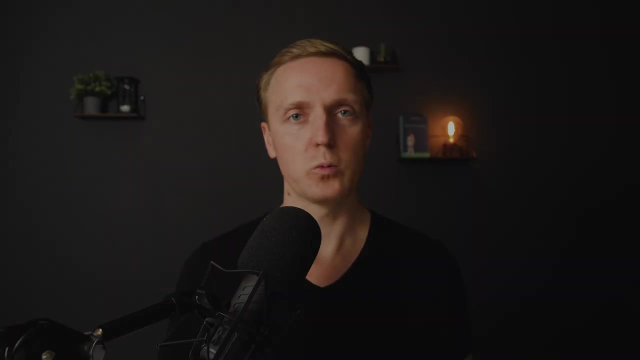 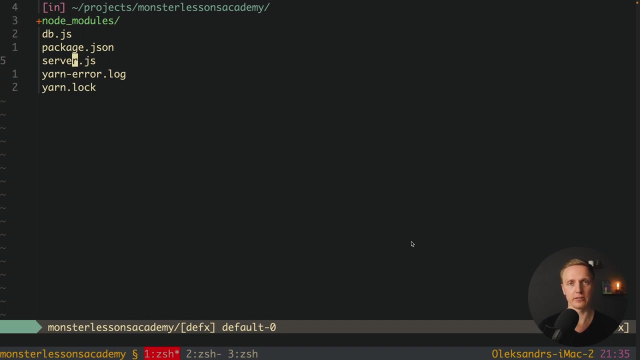 works, But obviously it is super dry and it is not clear. This is why I prepared an example for you, so we can implement the JVT token from scratch in an easiest way. As you can see here, I prepared for you a small project And we're interested here in two files: Serverjs. Inside node we have an 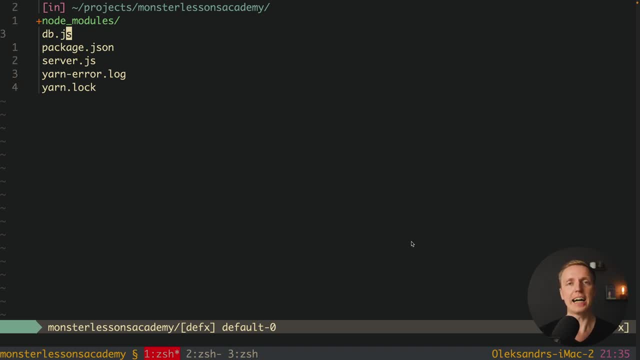 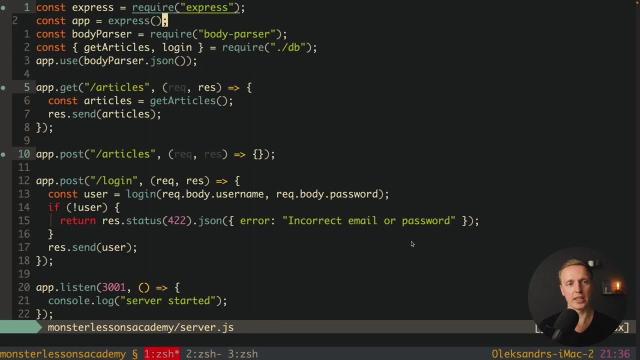 express server and a file dbjs, And here I don't have a real database and we don't need it Because essentially, it should not matter for you what database we are using, how we authenticate a user, because we implement JVT on top of that. So let's look on our server chest. As you can see, I have 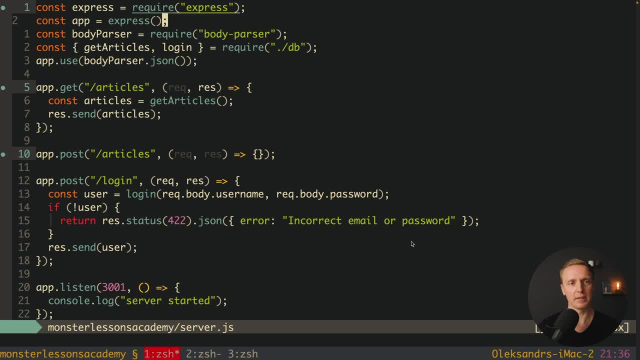 here quite a lot, but this is just plain express server. So first of all, here we have our express server and we have several routes. First of all, here we are getting appget slash articles and we are getting here get articles from our db. As you can see here on the top, we are requiring: 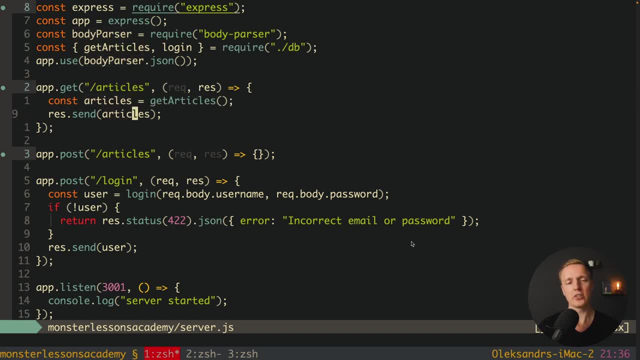 get articles from our db, And we are getting here: get articles from our db And we are getting here get articles method from our database And we are just sending them back. So let's check if it's working. I have our web server started on the port 3001.. Let's open postman and send request. 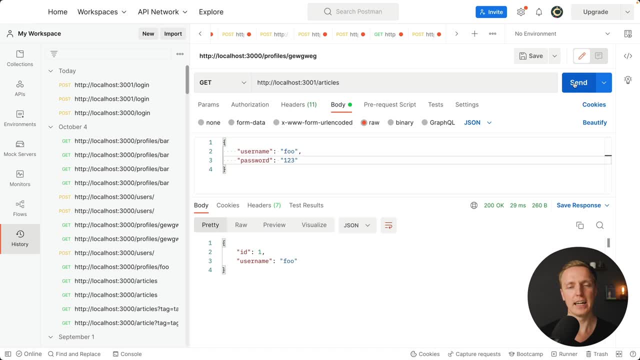 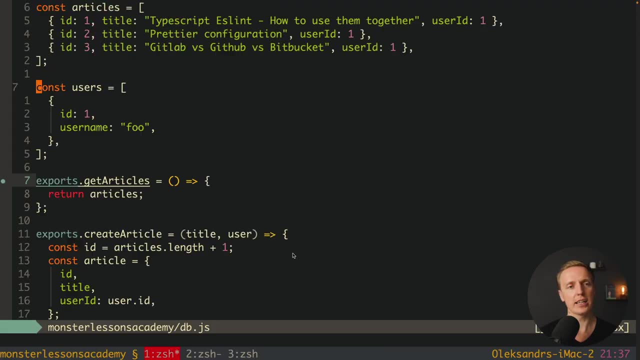 to slash articles- And this is a get request. I'm hitting here- send and we are getting back three nice articles. So what is that? Inside our dbjs, we have several methods. As you can see on the top we have some articles which are just defined. As you can see, here we have some articles. 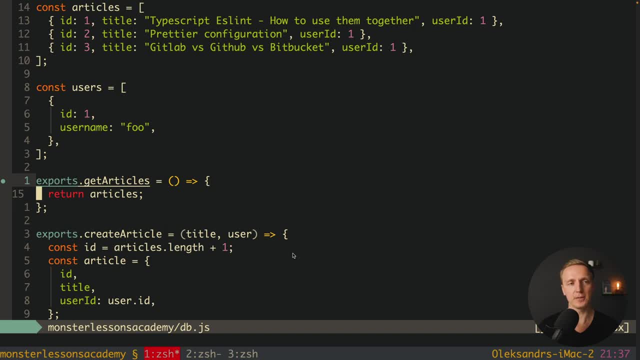 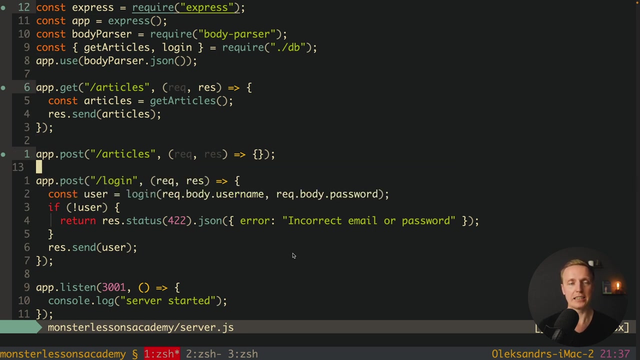 an array and our get articles method simply returns fast articles. Because fast, it doesn't matter how this db file implements storing of data or working with the database. After this, inside our serverjs we have a post request to articles Because we want to create a new article, but we 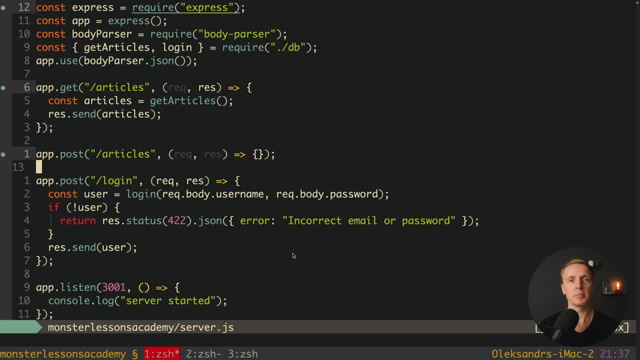 don't have any content inside this function. This is because we will implement it together to make an authenticated request to create an article. After this, we have a post request to login Where we are logging in our user with request body username and request body password. 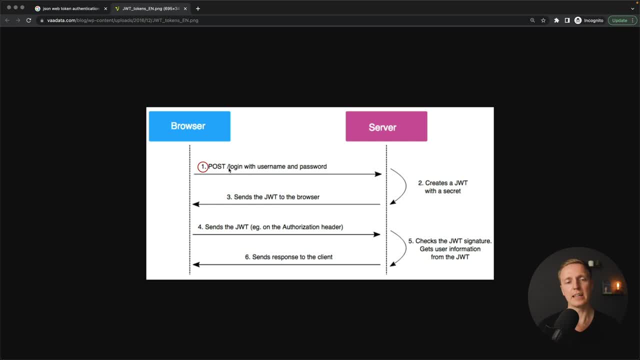 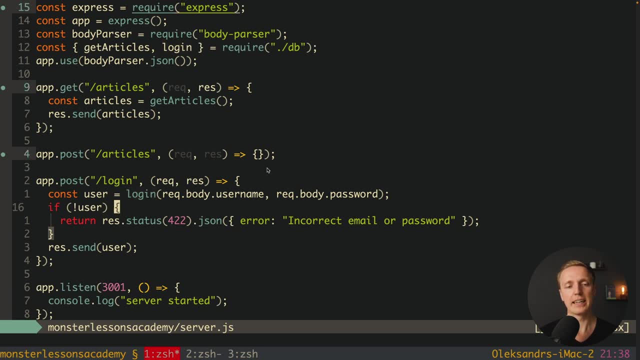 This is exactly what you saw on this diagram. We have here a post request with username and password, And if, after calling this login function, we didn't get a user back, Then we are throwing an error. In other case, we are responding with this user. Let's check what is login method As. 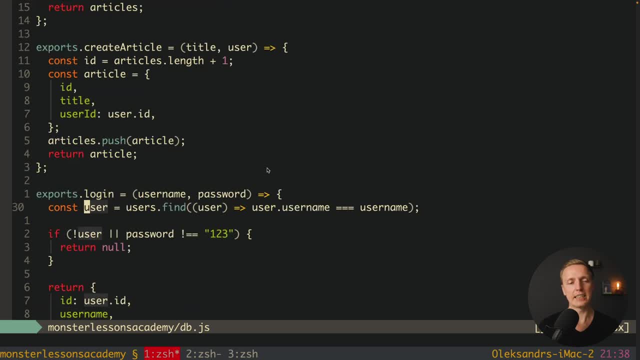 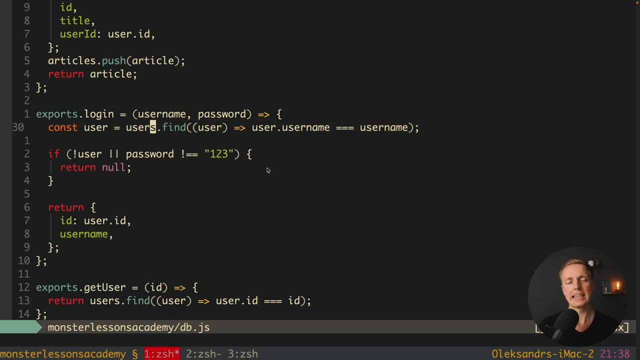 you can see, this is a function inside our db file And here is how it looks like. So this login is getting username and password And we are just trying to find a user inside an array of users. So what is the array of users here on the top After our articles? we are 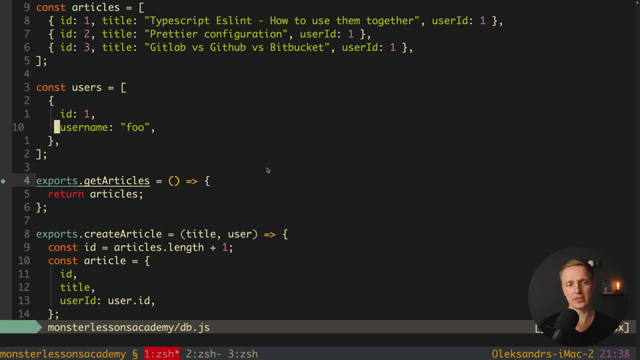 getting just array of users with id and username And, as you can see, here we have a reference between our users and articles. In every single article we have a user id and this is the author of this article. This is exactly how we typically store our information inside. 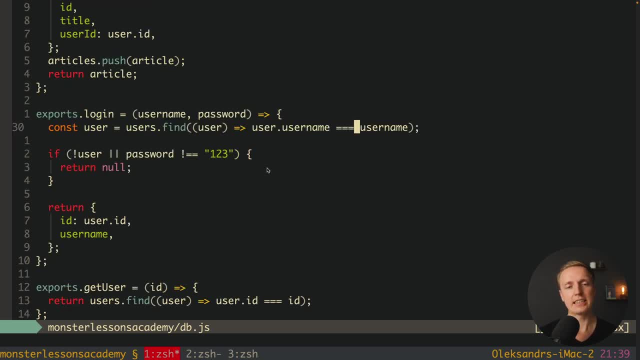 the database. So what our login method does? It tries to find the user by the username that we provided, And after this we are checking. if our username is correct And here our password is 123. Then we are returning user. If we don't have a user or password is wrong, then we simply 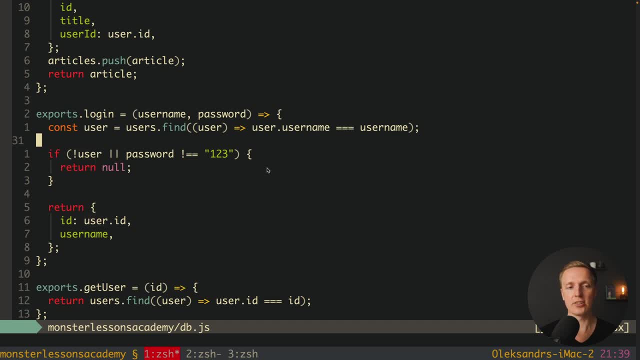 return here null, And in the real application, in such login function you will typically first of all get a user from the database and then check its password. But it is not related to gvt at all, Because we are using gvt after getting user information from the database. 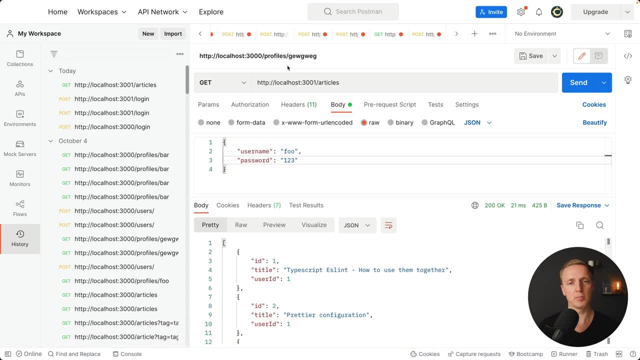 So let's check if this login function is working. I am jumping to postman and I want to make a request to slash login And this is a post request with such information. We have an object with username foo password 123.. I am hitting here send and we are getting back our user with id and username. This is. 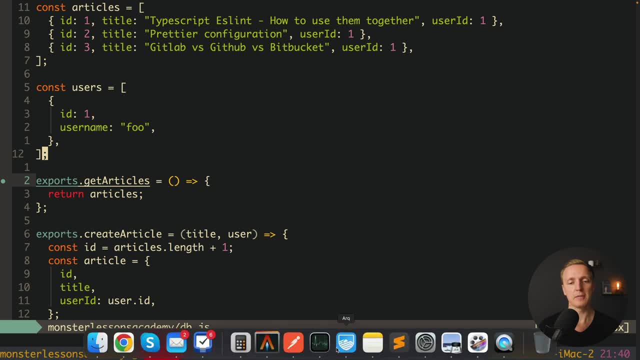 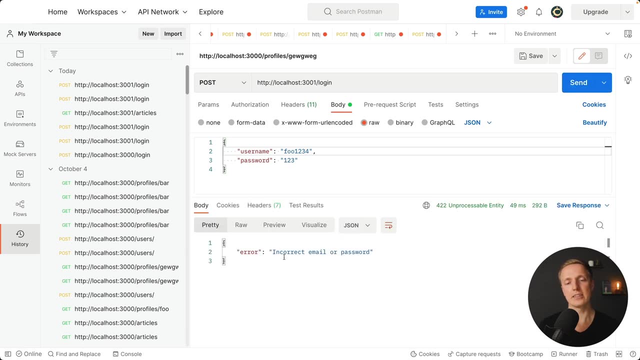 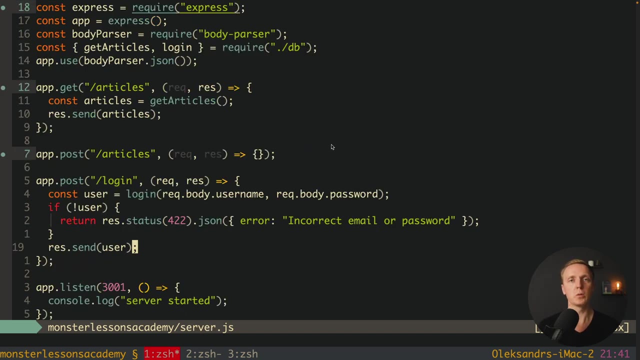 exactly the only user that we have here on the top If we are providing here some other information, For example foo 123.. I am hitting here send, and we are getting incorrect email or password. So our login function is working correctly. So now, on top of this small application, we must implement json web token authentication. 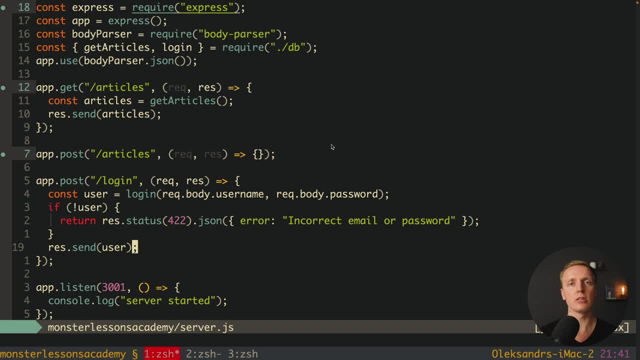 How we must do that. The first step here is to tune our login function. As you can see here we have a nice post to slash login. We are getting some credentials and we are checking here for the user. The main idea is that we must send back our user. 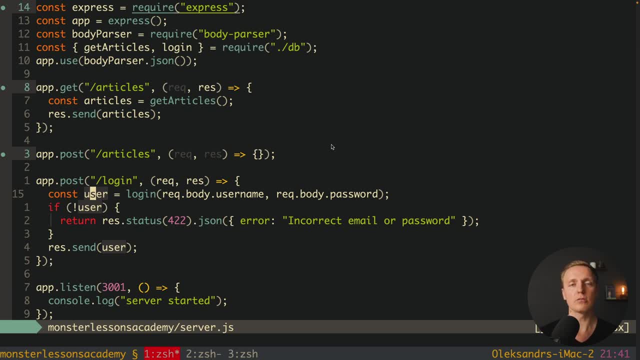 And we are checking here for the user. So we are getting back not just a user but also json web token. This is exactly the step 2, where we are creating jvt token, Which actually means we must jump inside this login function and create here a json web token. 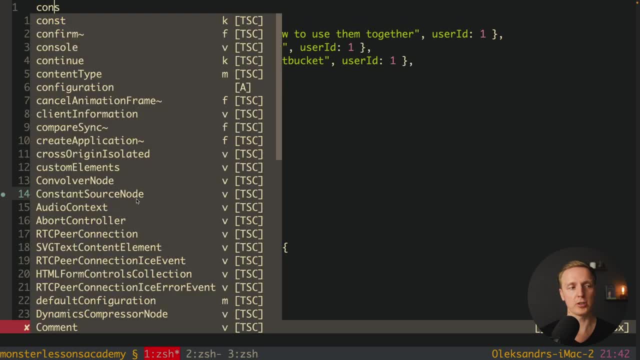 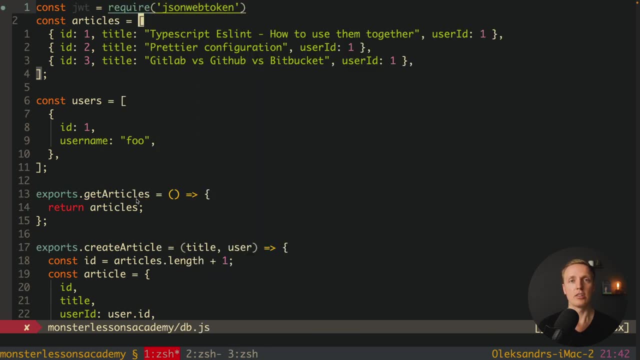 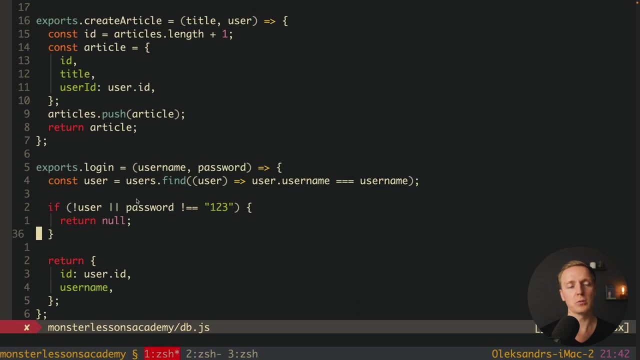 And for this we must use a library which is called json web token. So here on the top I want to create a property jvt and require this library, json web token, And obviously you must install this library with npm install json web token. So we are getting here GVT and now we want to use it here inside login function. 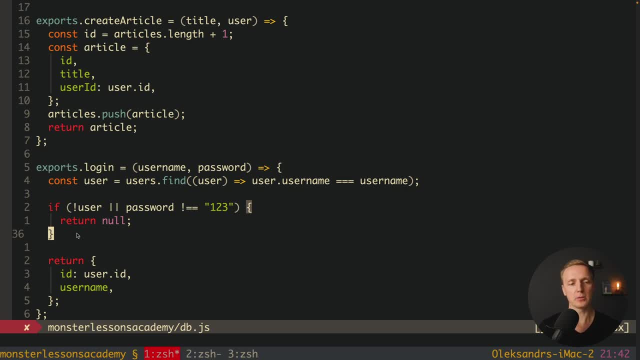 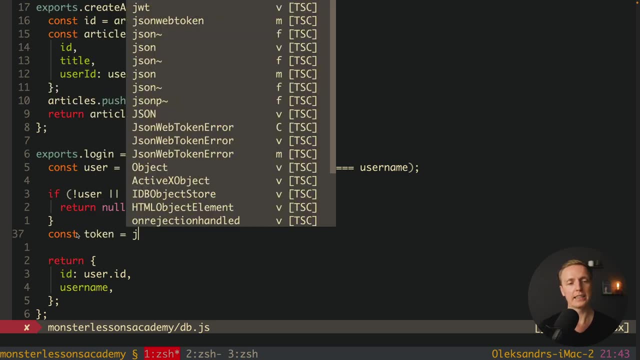 So, after we are sure that we checked a user and we checked it password, we want to generate a token string. This is why, after our if condition, I want to generate a token and I want to call here gvtsign, and this is exactly a function to create a token. 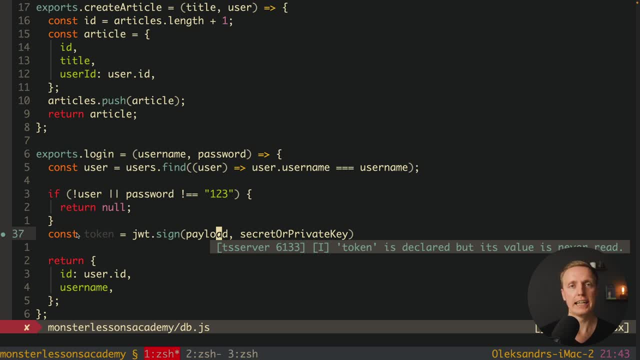 And here we are providing two things. First of all, our payload. This is exactly what data we must write inside our token, And typically we want to store inside an id of our user, Because by id we can always find a user from the token and understand what user sent us the token. 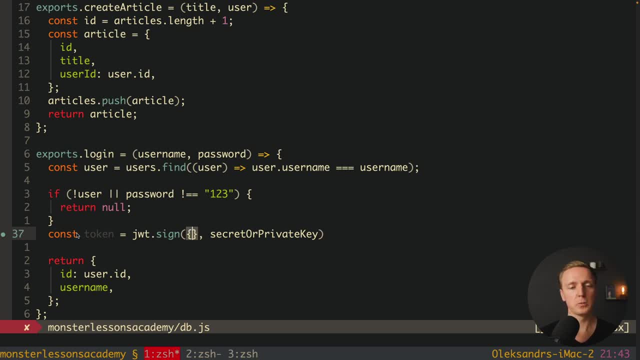 This is why here inside payload, I want to provide an object with field id and in our case it will be userid, and also we can provide additional username just to understand what user it is without getting it from the database. And now the question is: what is a secret? 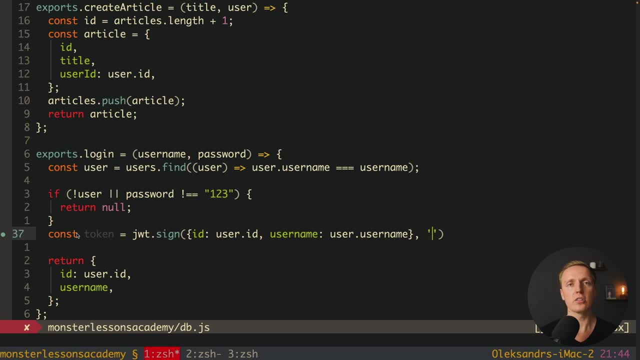 And actually this is any string on the backend which nobody knows. For example, we can write here full bar bus and this is totally fine. The main idea is that only with this secret string our backend can parse this gvt token back. This is why it is completely safe to send gvt to the client. 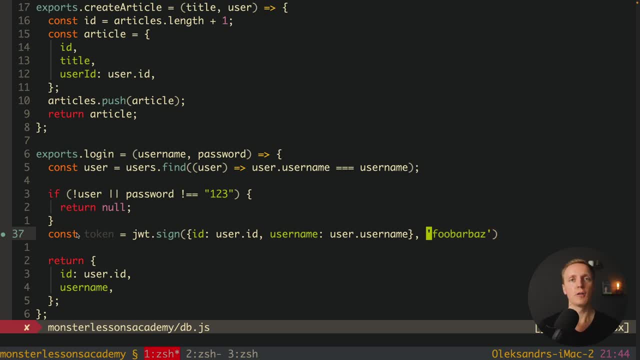 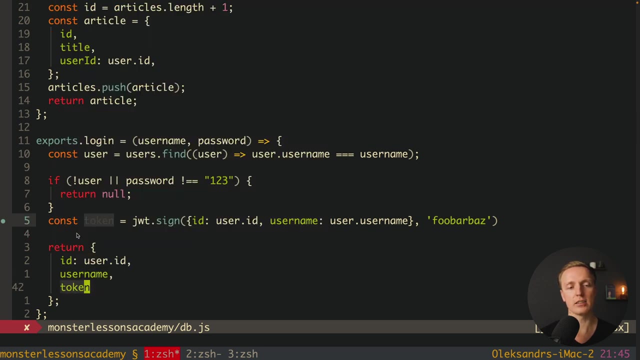 and nobody can understand what user was that. So for your project, it is extremely important that this string stays secret and nobody ever gets it. In other case, you can leak user info. So here we are, generated our token, and now I simply want to add this token to our response. 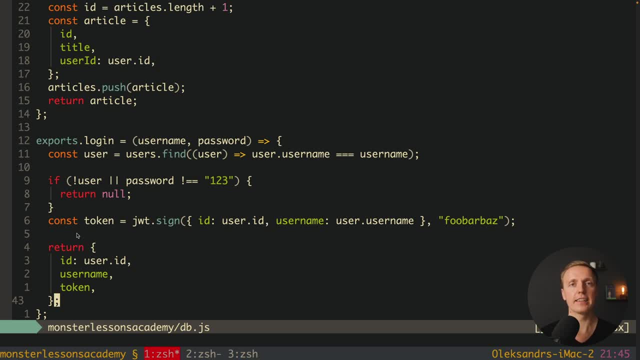 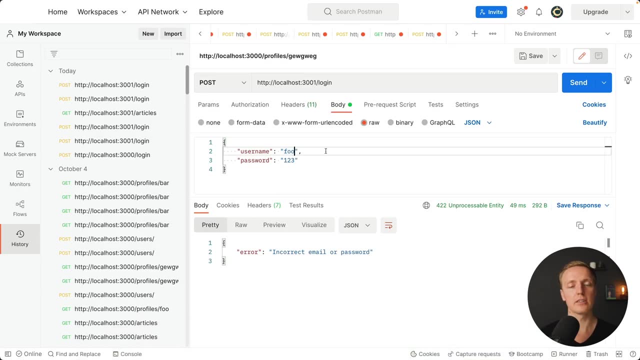 In this case we are directly sending, after logging in, this token to our client. Let's check if it is working. I will jump back to the postman and here I will login with correct credentials. I am hitting here send, and we are getting not only id and username, but a new token field. 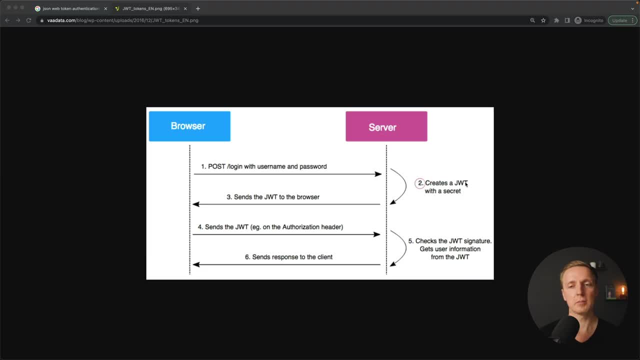 And, as you can see, this is just a string. As you can see, we implemented step 2 with creating a token We are creating of our gvt secret and sending it back to the browser. Now, after we responded with this token, our client must save somewhere inside local storage. 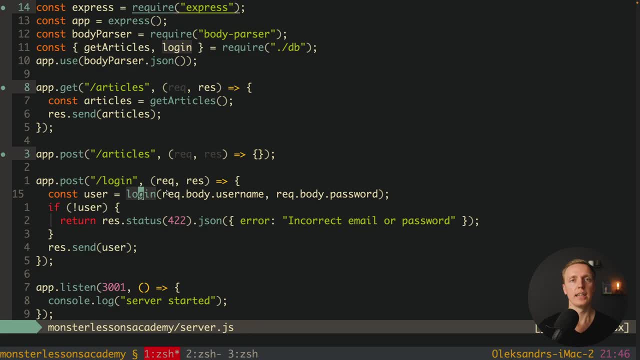 or a cookie, this token for the later use. And now we are coming to an interesting point: When our client will send for us correct token, we must parse it, check it, get user information from it and respond with the correct data. And for this we will implement this POSTARTICLES function. 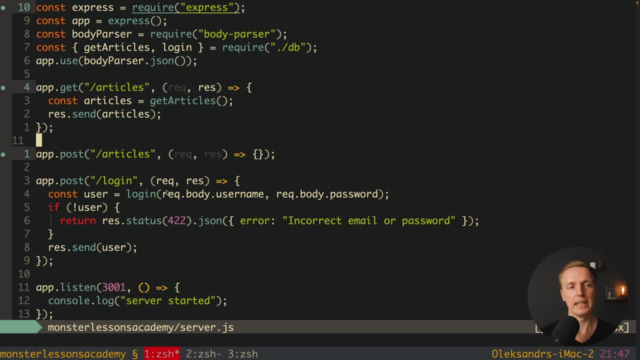 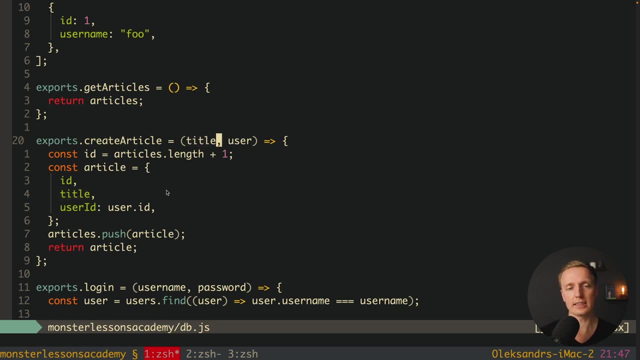 And only correctly logged user can create an article And as you can see, here inside dbgs we already have a function- createArticle- And we expect here to get a title of the article and the whole user. And actually this whole user is not coming from the client. 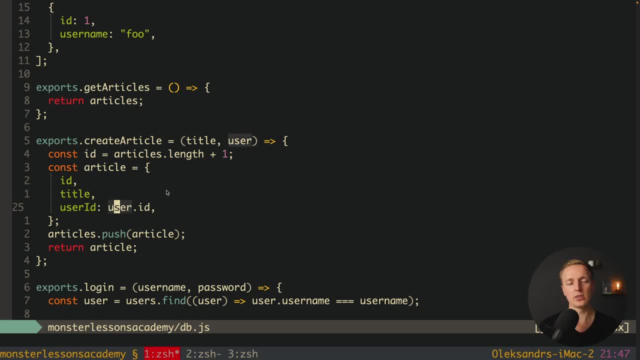 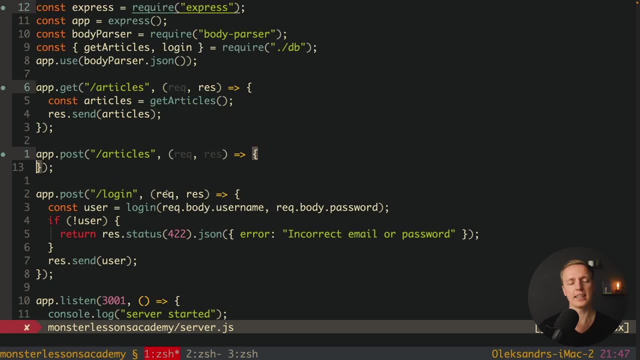 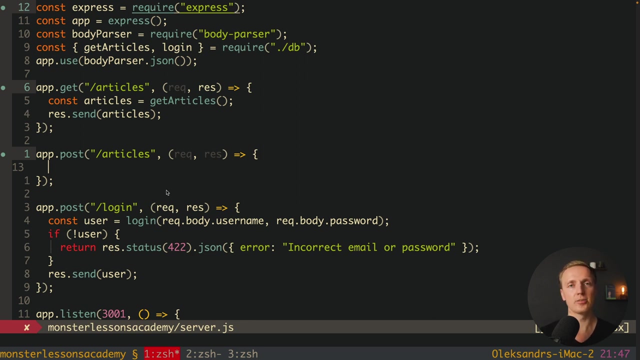 Our backend must get it, Because here we are using userid information to create a new article and push it to our array. So actually, what we could do here inside our POST for articles, we can directly from our request, read all headers, parse them, then get user information and do some logic. 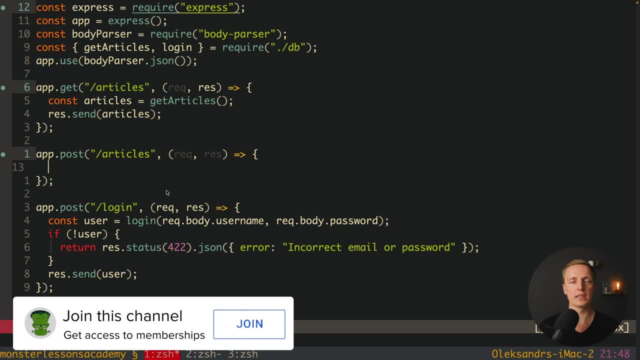 But this is a bad approach. Why is that? Because, actually, we will need exactly the same code in every single place where we want to authenticate a user. This is exactly why do we want to build authentication middleware. So what is authentication middleware In express, before we are getting to this function, this callback of any route we can actually 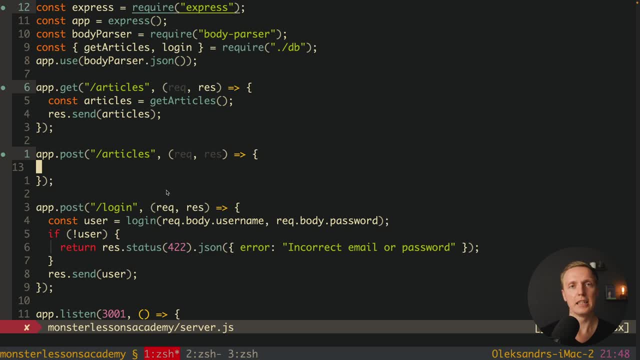 call a middleware, And this is just a function in the middle between starting of our request and coming to this function to respond. We can just do there some logic, And this is exactly the place where we want to check if user is logged in. if we need 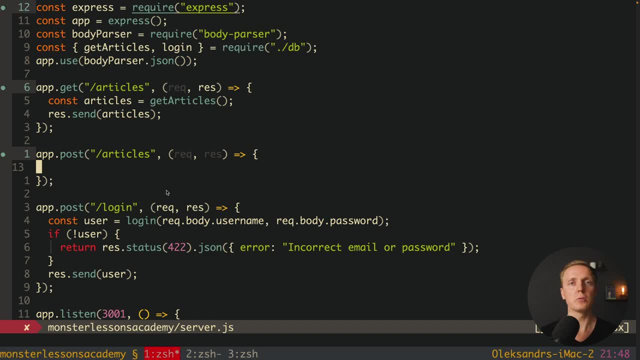 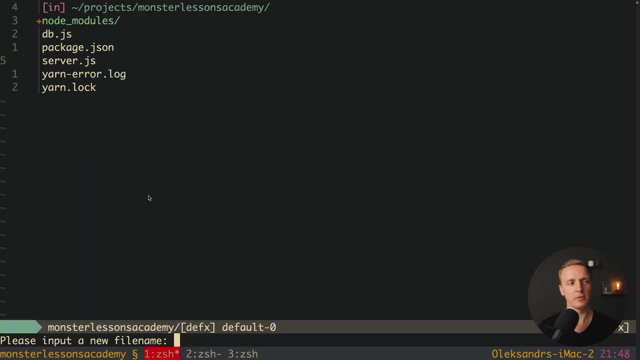 to send 401 back and he is not logged in, Or where we need to parse our JSON web token. This is why let's create now a middleware. So for this I want to create a new file which is called althmiddlewarejsp. 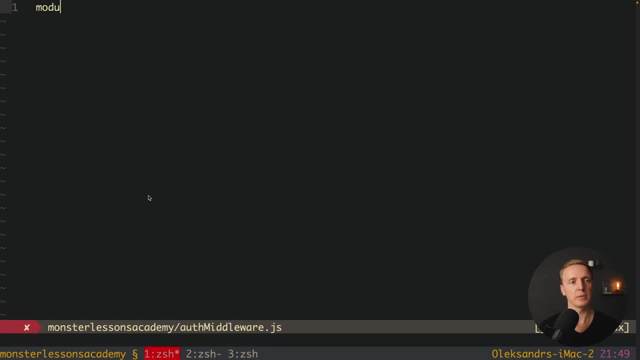 And now in inside we create just a single function. This is why here module exports And here we are getting request response and next. And next is important here, because after our middleware is finished we are calling next And then we are saying that our request is ready to be continued to our route function. 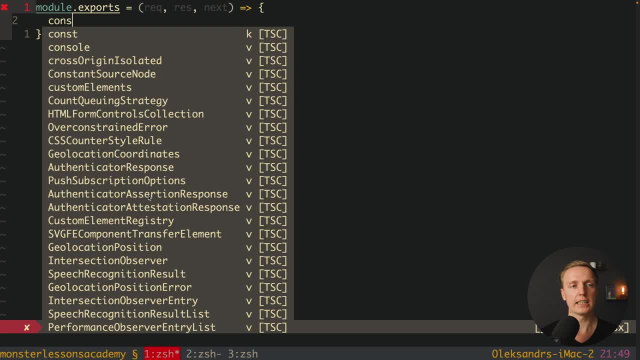 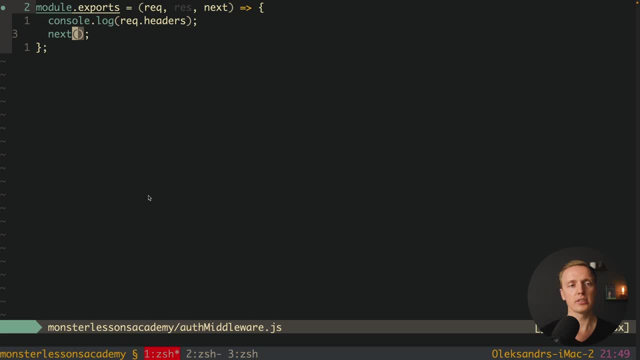 So first of all, let's check if it's working at all. What I want to write here is consolelog request headers, And after this I just want to call a next, Because in other case it won't work. Now let's use this althmiddleware inside our serverjsp. 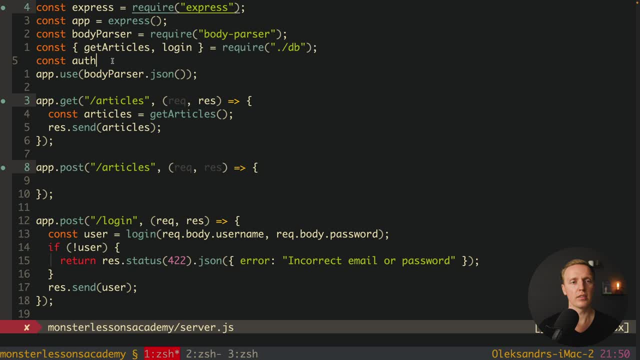 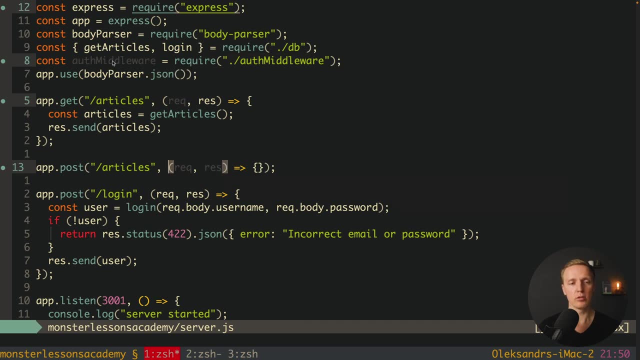 First of all, here on the top, we want to get this althmiddleware from the file that we just created And it is althmiddleware. Now, here inside our post for the articles just before our function, we want to write althmiddleware and then comma. 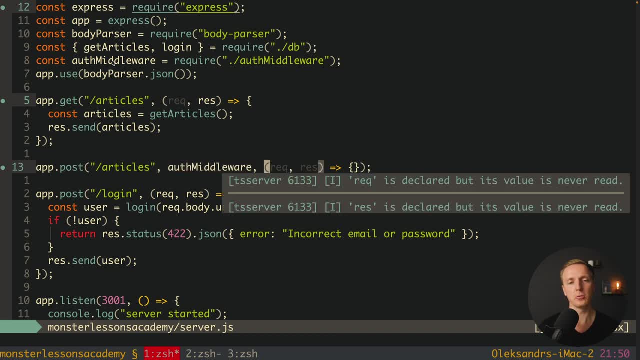 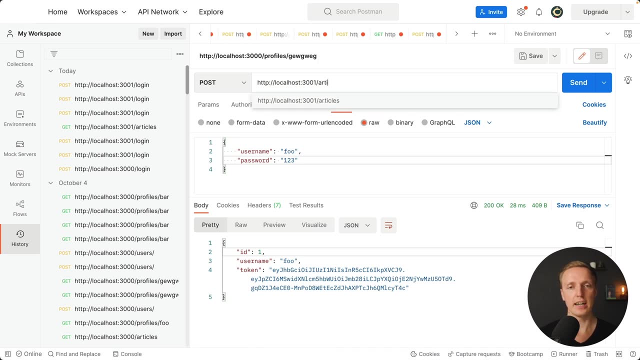 And it means that we are calling this althmiddleware. before we are coming to this function, Let's check if it's working For this. I want to jump to postman and write here slash articles and this is a post And for now body doesn't matter. 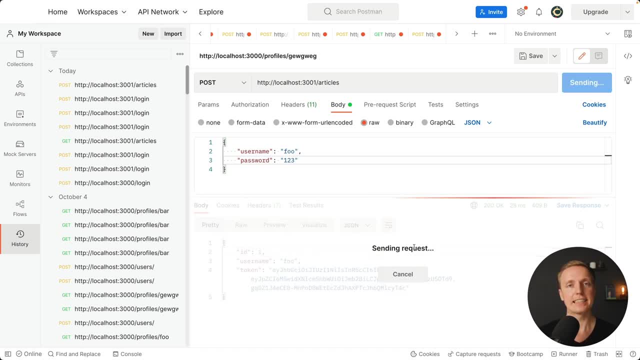 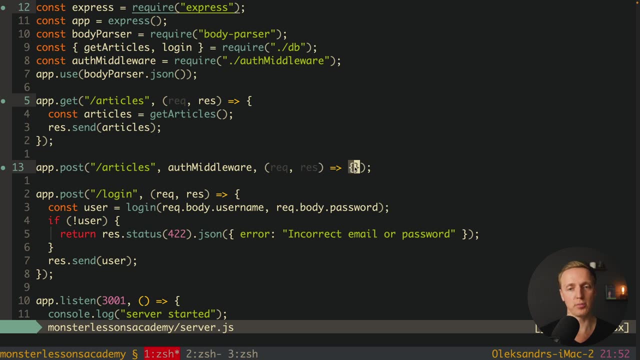 I'm hitting here send and we are getting sending request And this is a pending request Because we didn't write inside our function- post articles- any code with response. This is totally fine, But as you can see here inside our consolelog, we are getting this object. 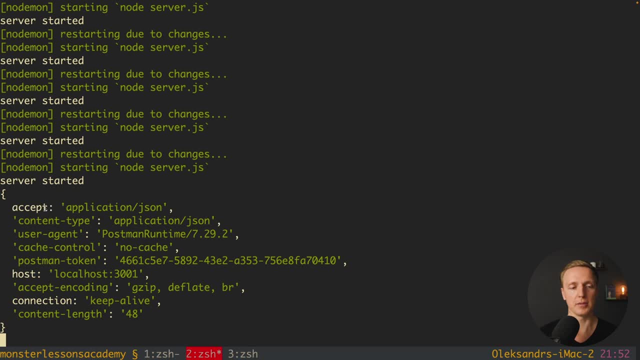 And this is exactly all our headers that we provided from the server, And this is exactly all our headers that we provided from the server, And this is exactly all our headers that we provided from the server. So what I want to do now, first of all, is write a response. 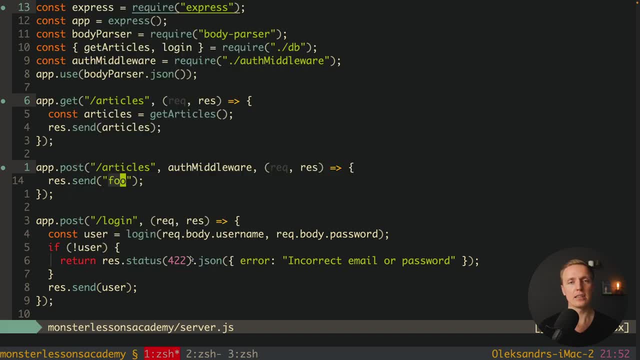 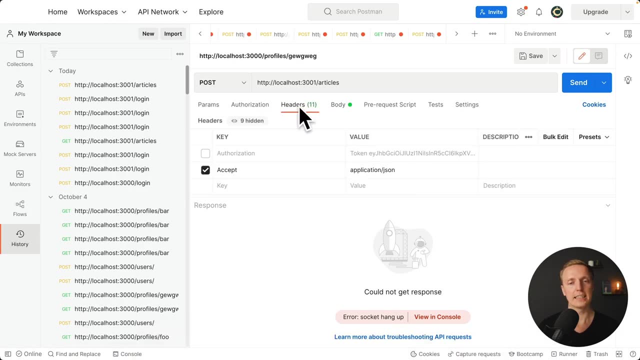 This is why here let's write res, send, for example, full, And also I want to send some headers that we really need to check. This is why I will jump inside postman, inside headers property, and here we can add a new key which is called authorization. 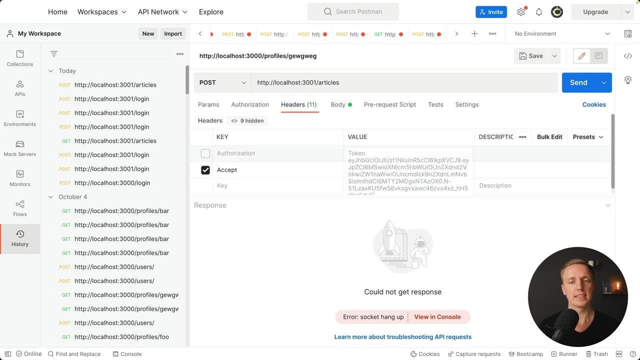 So here, as a key, I will write authorization, and as a value, it must be our token. And just to remind you, I copied the token from our althmiddleware. This is why now I will paste it here, Which actually means we added to our headers a new authorization token with such value. 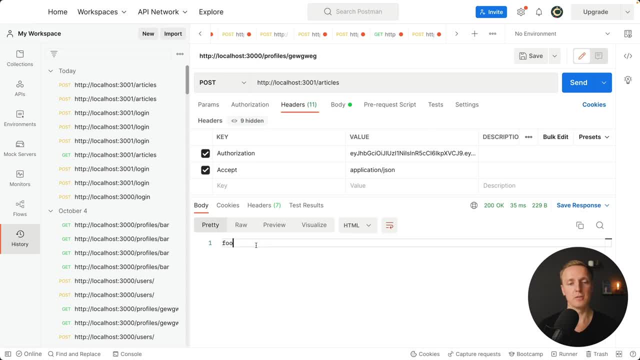 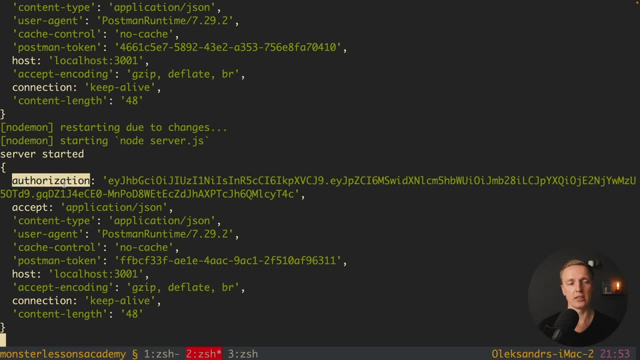 Now let's send this request again. I am hitting send and we are getting full. This is totally fine. And here inside console we are getting our headers And here we are getting authorization token And this is exactly the value that we want to get from the client to authenticate our 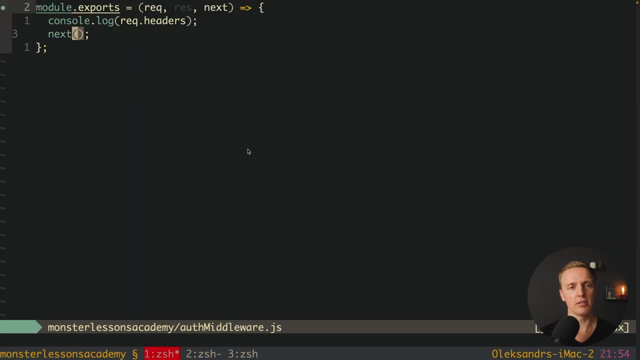 user, So let's use it. now We want to jump back inside our althmiddleware And we know that we have our value inside request headers, So first of all we can try to read it. So here we are getting our alth header. 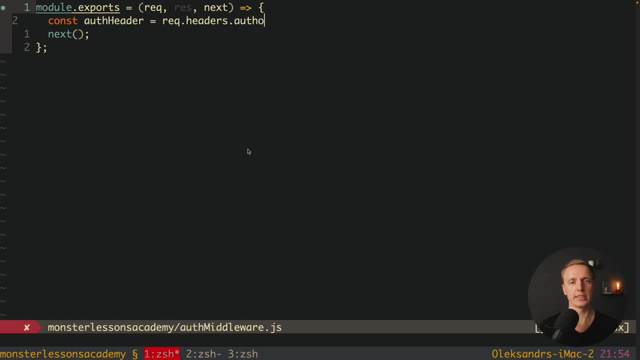 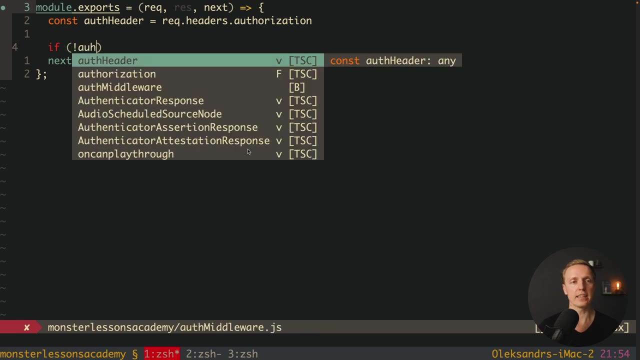 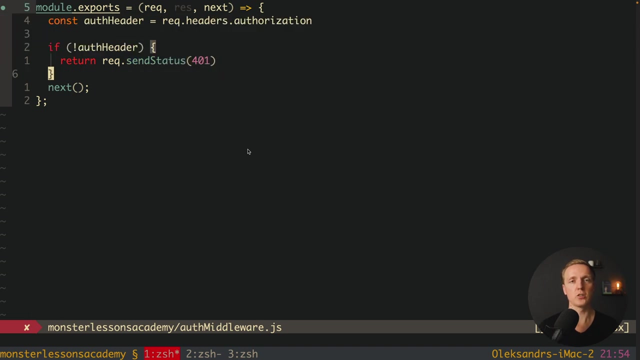 And this is requestheadersauthorization. If we don't have this header, it means that we are not logged in. This is why here we can say: if we didn't get our alth header, we want to return res, send status And we are sending for 01.. 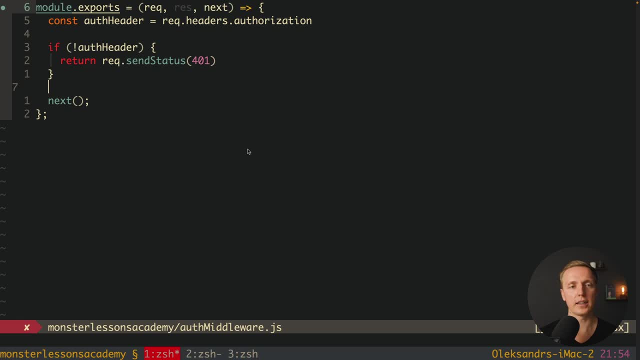 Which means unauthorized. After this we want to try to parse our token. This is why here on the top, we must require gvt library. So here I am writing: require jsonwebtoken, And now let's use it. So we are getting here back some data after we are calling gvt verify. 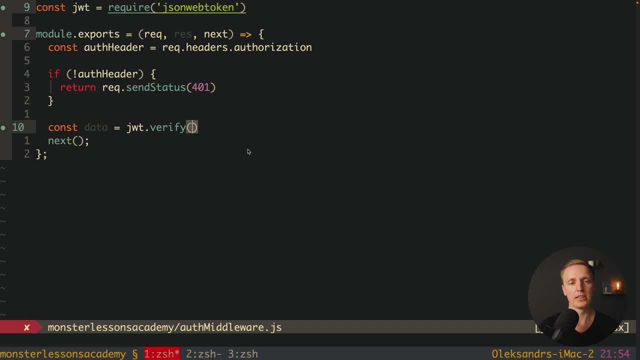 And this is exactly what we are using to check our token. So, inside our verify, first of all we are throwing our header And secondly our secret. And, just to remind you, Inside our dbjs, inside our login, we had such secret And I will just copy it. 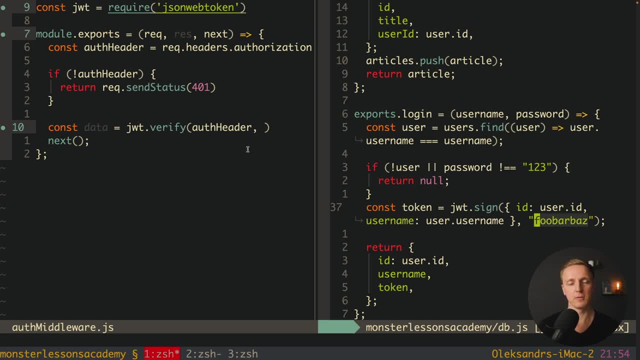 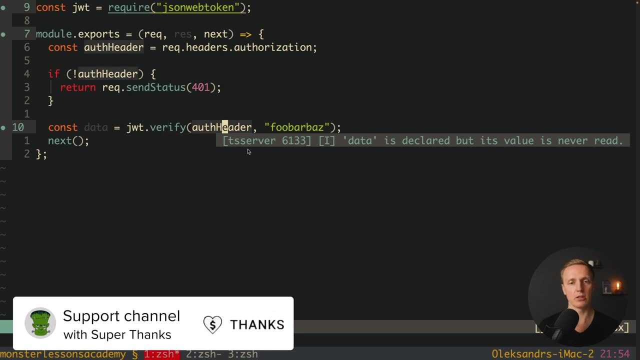 You can obviously put it in some constants And share between two files, But for the sake of testing I will simply paste it here. So inside our verify function we are throwing our token And secondly, our secret key, which we know only on the backend. 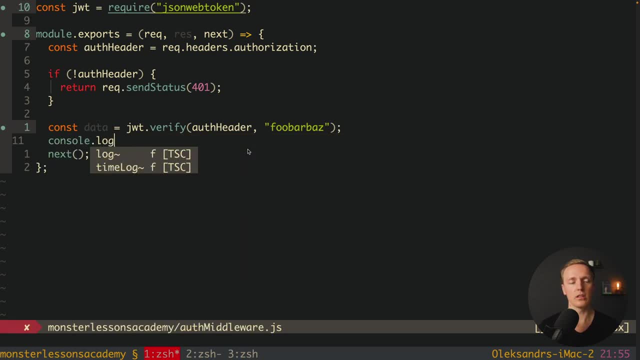 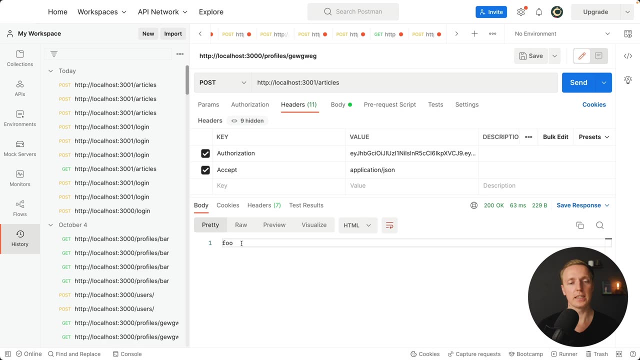 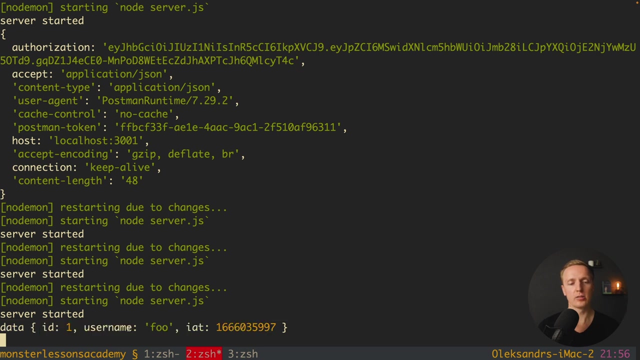 And we are getting back some data. So now I want to console log what data we are getting and check it in the console. So here let's hit send again And, as you can see, we are getting foo. Everything is fine. And now inside our data we are getting an object with id 1, username: foo. 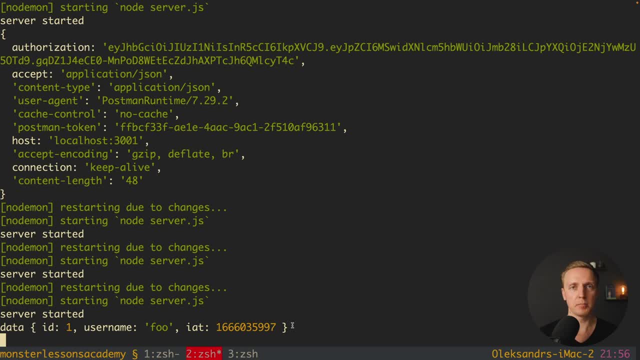 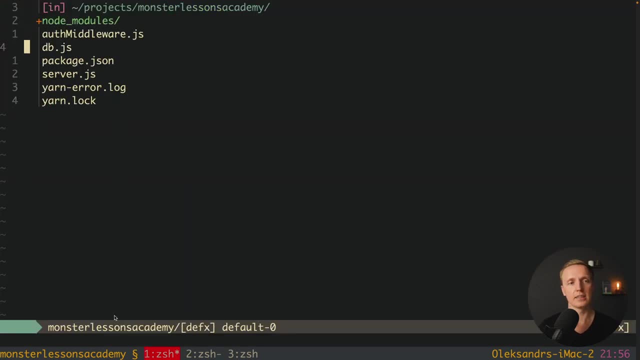 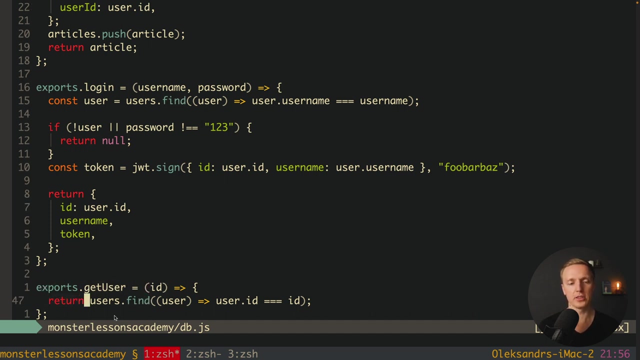 And here is the timestamp, Which actually means we successfully parsed our jsonwebtoken And now we have enough information to get a user. And for this inside our file dbjs we have a function at the bottom Which is called getuser. And here we are getting from our ref users. 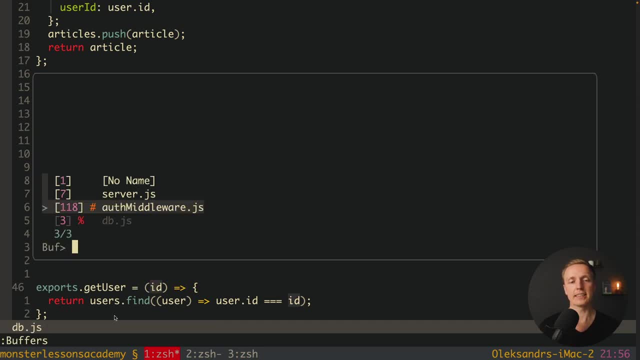 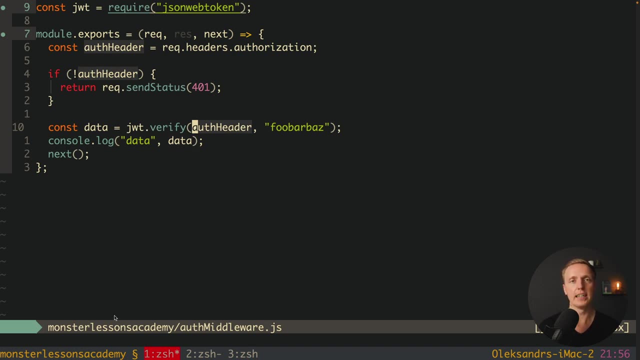 A user by default by id that we provided inside, And this is exactly how you want to write the code inside a middleware. In the real application. you will make a database request here to get a user by this id. In our case, here we can simply use the function getUser. 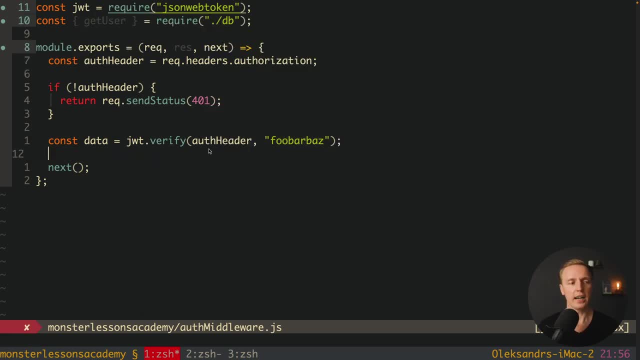 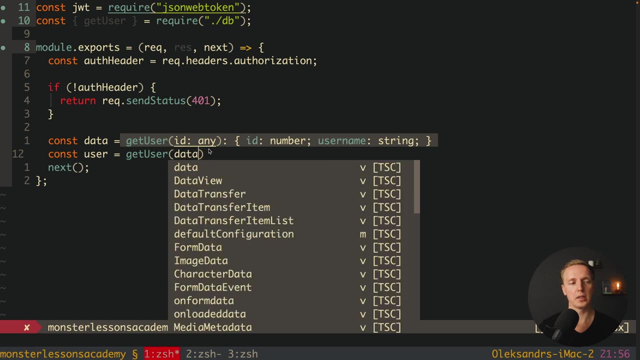 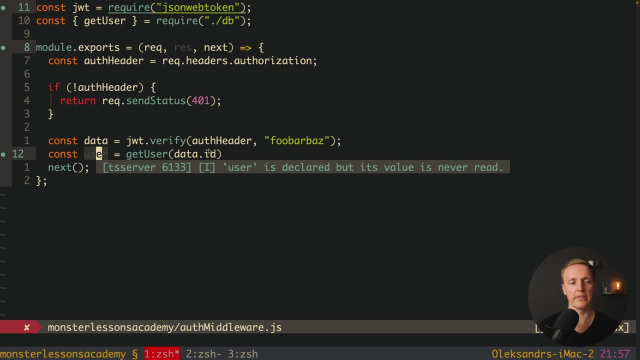 And we are requiring here our db file. So here, after getting our data, we can get a user, And for this we are calling our function getUser, where inside we are pasting dataid. So this will for sure get for us a user, because we know that it was a valid token. 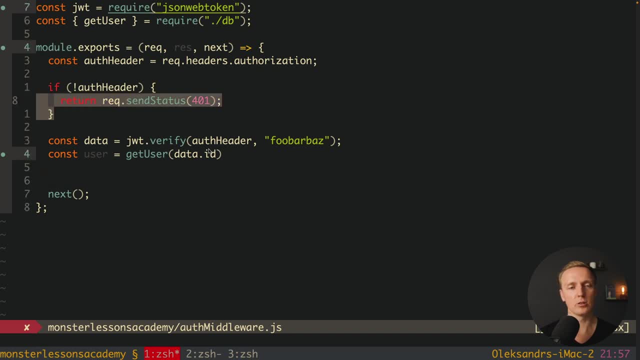 But if you want to be on the safe side, you can just copy paste this code with if condition: And if you don't get a user from the database, then you just respond with 401.. In this case, if for some reason you are not getting a user, you will still be on the safe. 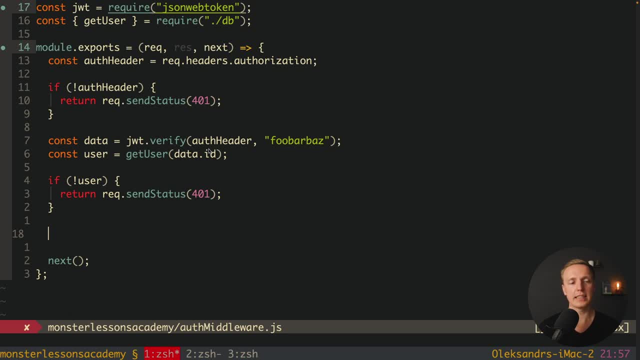 side And the last step here that we want to do: we want to update our request So we can read a user later inside our application. And for this we can see that we have a user And for this we can see that we have a user. 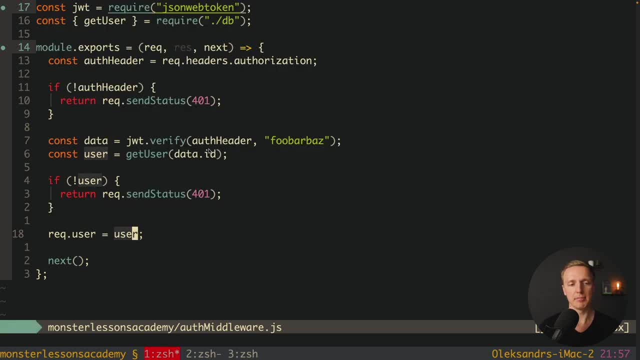 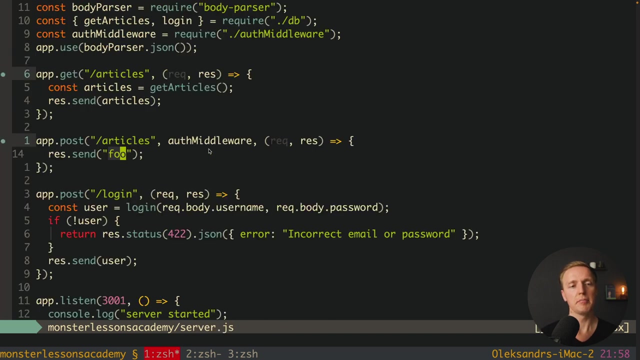 So we simply write: requestuser equals user, And with this line we simply updated our request so we can read user information later inside the function. And this is exactly how we implement middlewares inside express. Now let's jump back inside our serverjs, because now, instead of this resend, we can create an. 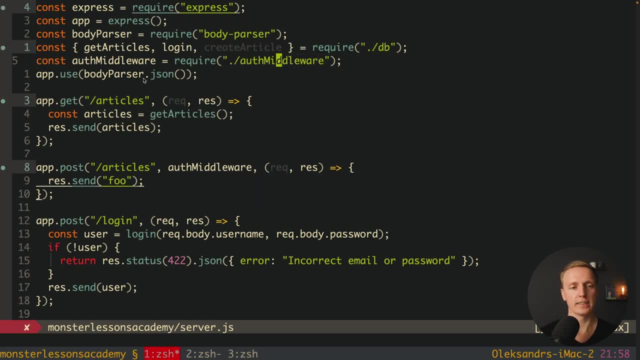 article. This is why here I want to import createArticle function. Now, here, instead of resend we want to create new article. So here let's create a property article and we are calling here createArticle function, where inside we must provide first of all requestbodytitle. we are reading it from: 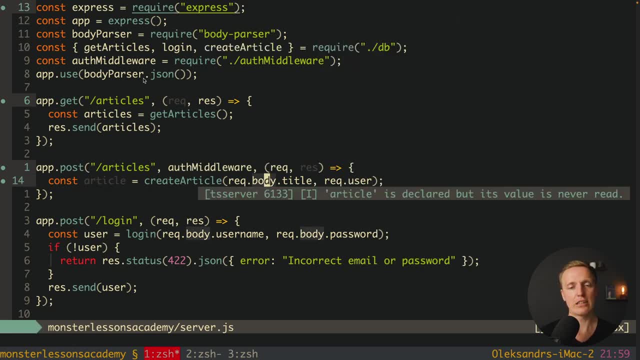 the body and secondly, requestuser. And just so you fully understand, we are not getting this user from the client. From the client we simply get a token. but because of this auth middleware we got the user on the backend and now we can use it inside our function from requestuser. 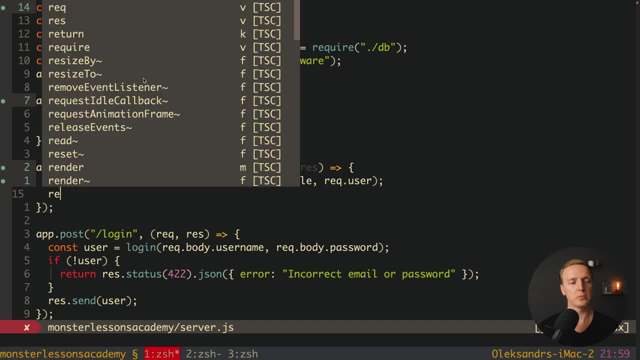 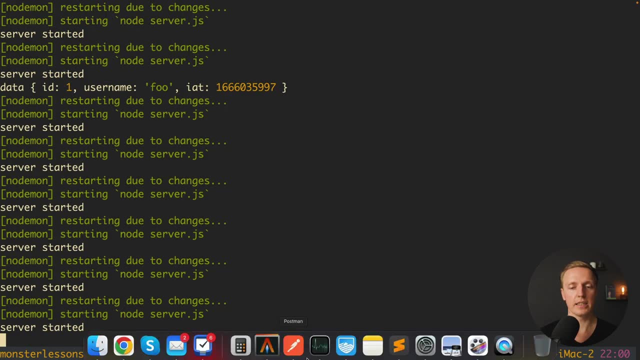 So this single liner will create for us new article and we can just respond with resend. and here is our article. Let's check if it's working. As you can see, we don't have any errors. and now I want to create a new article. 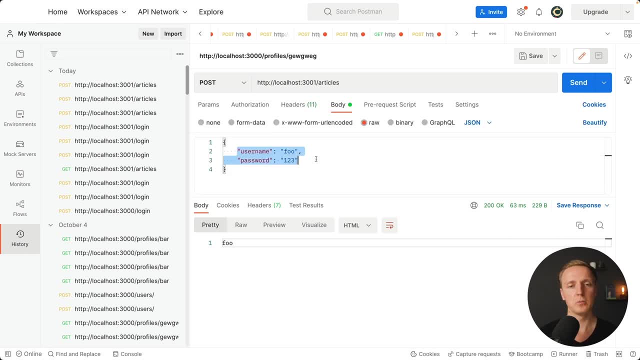 So it must be a POST request and here inside body we must have just a title property. For example, let's create a title GVT. I am hitting here send and, as you can see, this is our response. we are getting here id fortitleGVT.